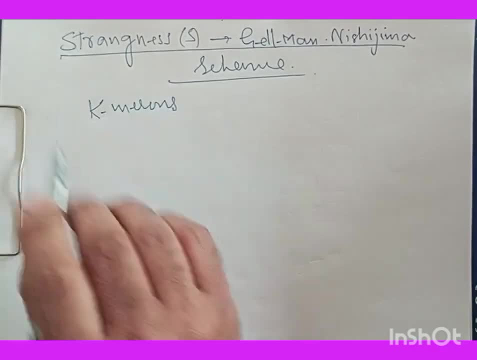 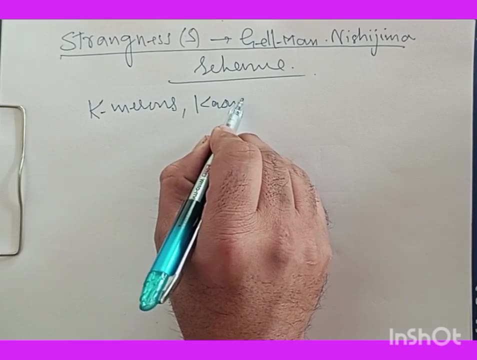 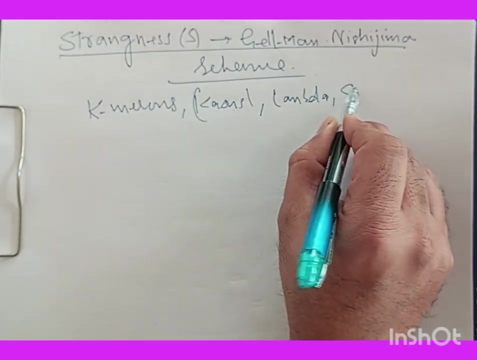 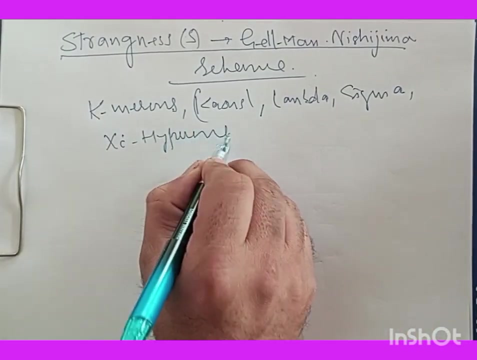 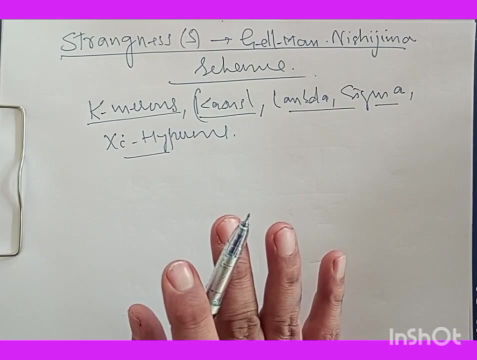 massons, or we may also call them as k-ons, lambda, Sigma, chi, hyperons, all of these particles are called a. I mean, all of these particles are called strange particles. and these particles are called strange particles and they have reasons for that. the very first important reason is that they are 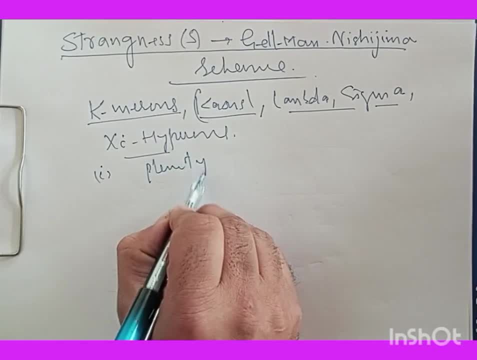 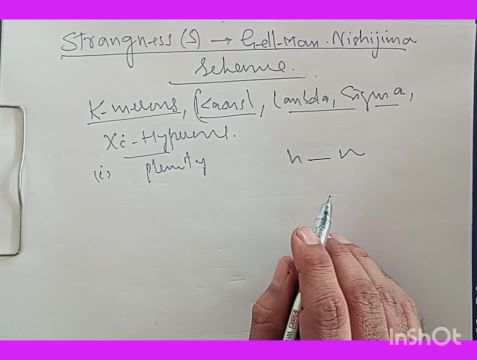 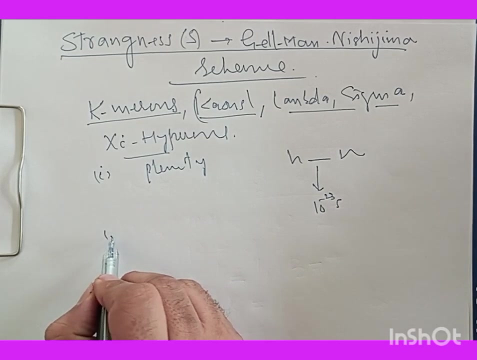 produced in plenty. they are produced in plenty through strong interactions between between nucleons, and and the and the and the collision time. here we know that this collision time is is very short, of the order of 10 to the power of minus 23 seconds. and the next important reason is that that they are always produced in. 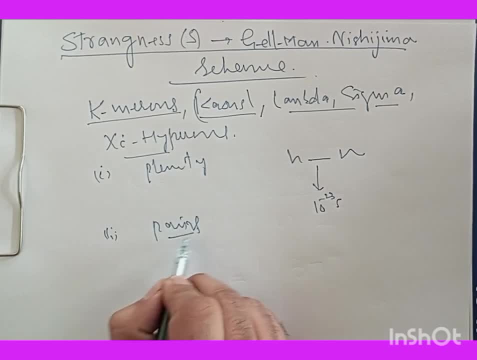 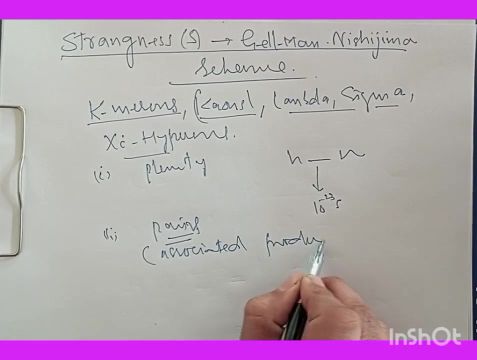 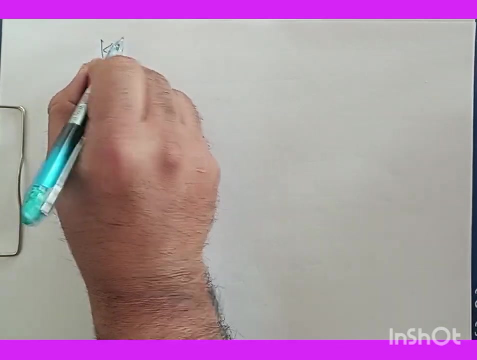 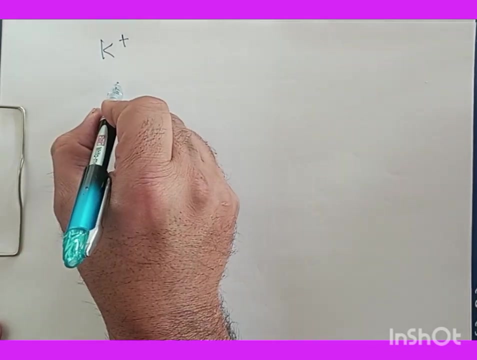 pairs. always, they're always produced in in pairs and this is also called as associated production. associated production and the next important thing is that they they decay reluctantly through weak interactions. so they decay through weak interactions. now, if i take an example of, say, if i take an example of K positive meson, and these mesons are produced in pairs as follows, suppose we 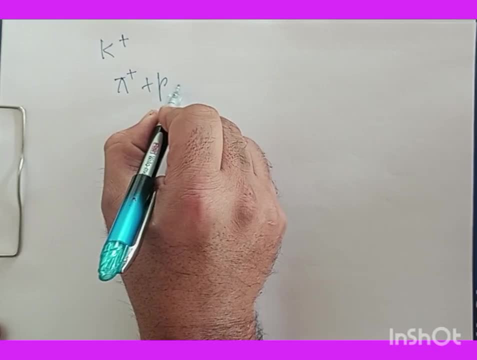 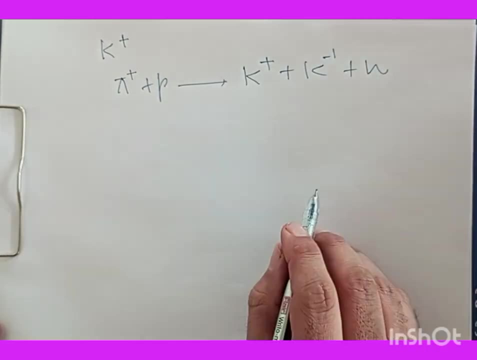 have pi positive meson and a proton. it leads to K positive plus K negative and a neutron, and this strangeness is related to the electric charge and it is related to I3, the third coordinate of isospin, and it is also related to the baryon number and there is a relation between this. 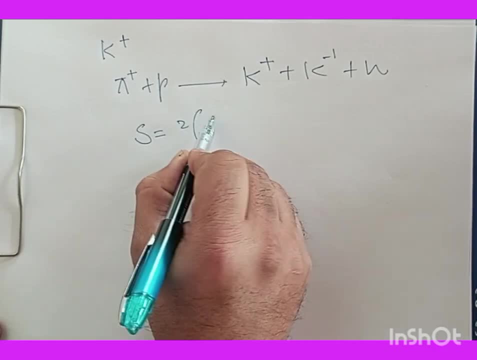 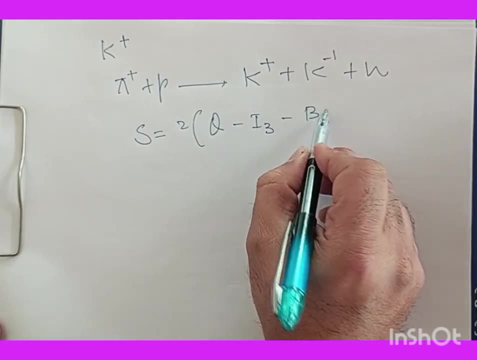 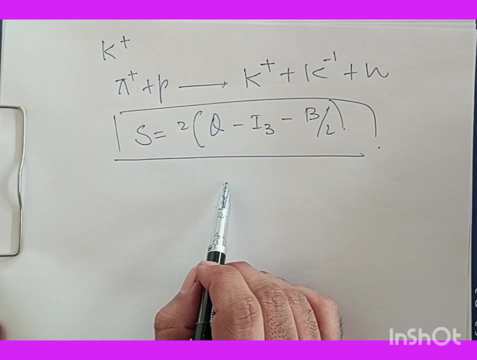 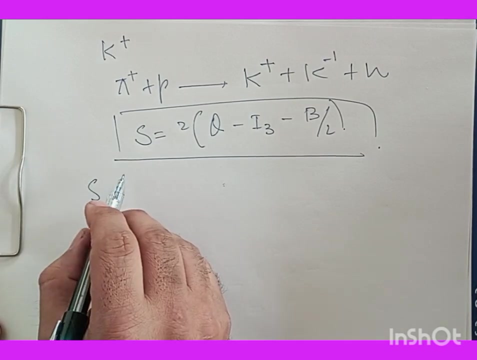 strangeness. and that relation is: S is 2 times Q minus I3, the third component of isospin, minus baryon number by 2.. Now, this is a very simple equation. Now, this is a very simple equation. Now, this relation is known as Gelman-Nishijima relation and this strangeness is non-zero. 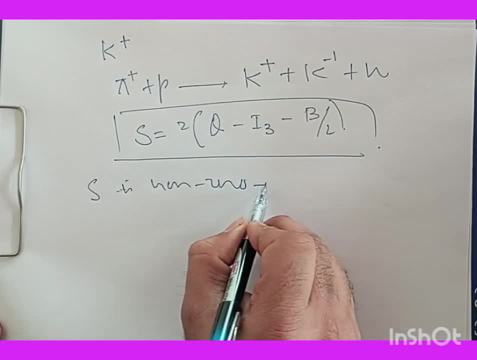 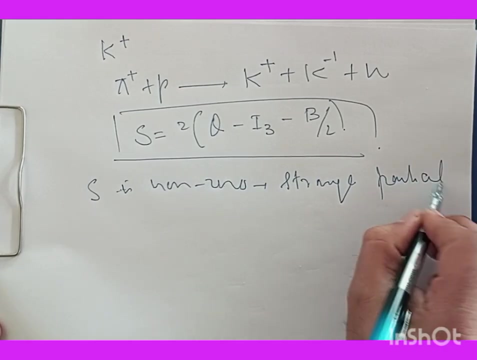 S is non-zero. it is non-zero for strong particles and, sorry, it is non-zero for strange particles. I should say it is non-zero for strange particles and and it is zero for all other particles, and I can say that this S is non-zero, it is. 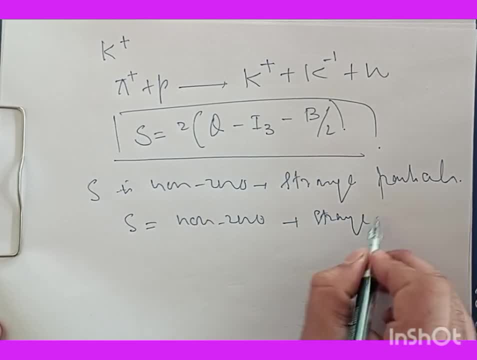 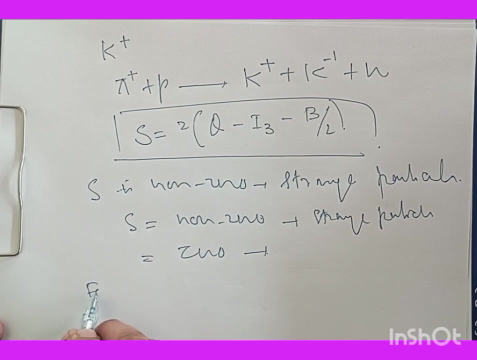 non-zero for strange particles, strange particles- and it is zero for everything else which are, which are not strange particles. now, if we have to calculate the strangeness of some of the particles, say if we have to calculate the strangeness of some of the particles we, for example, for for K positive, we want to calculate its strangeness, that will. 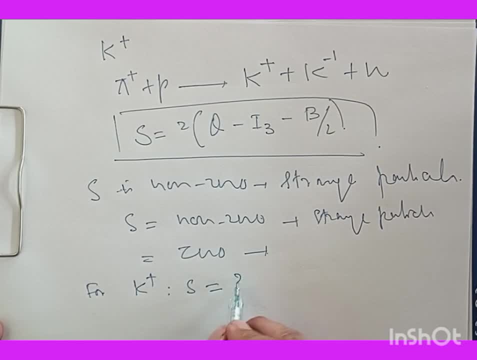 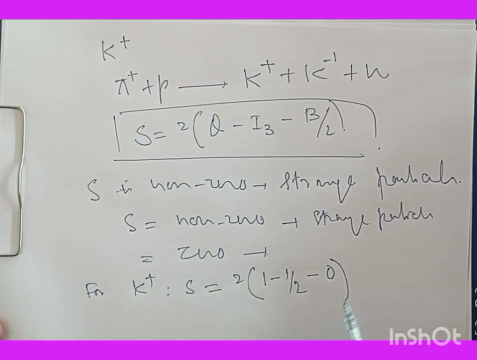 be. S is yeah, two times Q, that is one. okay, its third component of isospin is half. I mean it's minus half, and minus zero doesn't have any variant number. so it's strangeness is equal to plus one, and, and similarly we can calculate for: 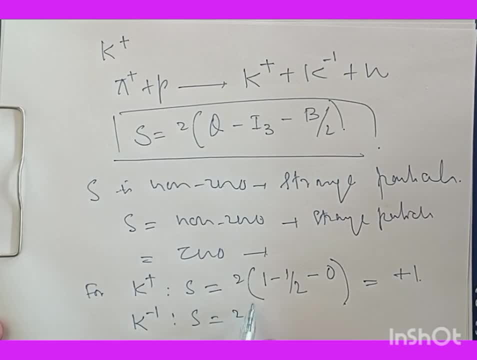 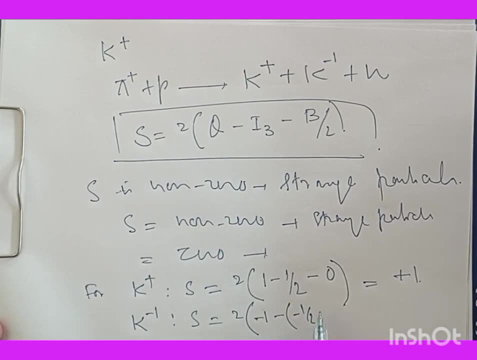 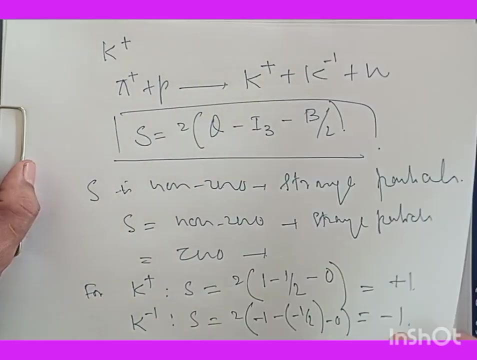 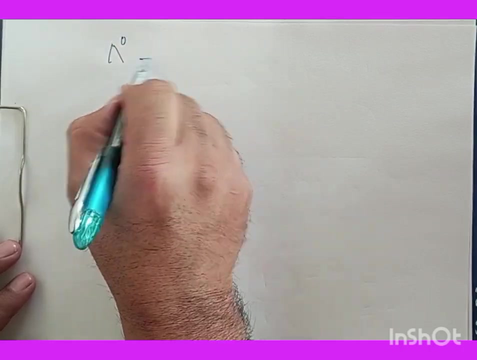 other particles, say K minus, the strangeness will be two times. it has minus one charge and it is minus times minus half and minus zero and this is going to give me minus one. and we can take another example. say: say I will take, take lambda neutral and for this particle strangeness will be two times, doesn't have any charge. it. 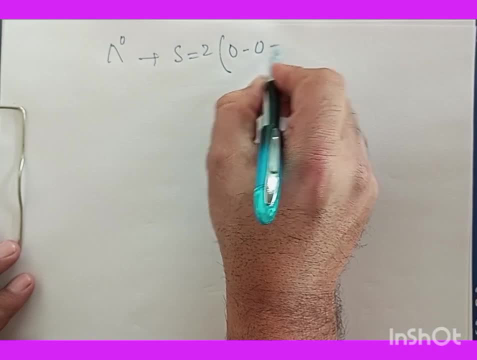 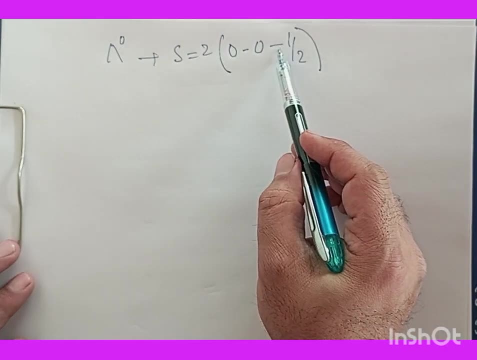 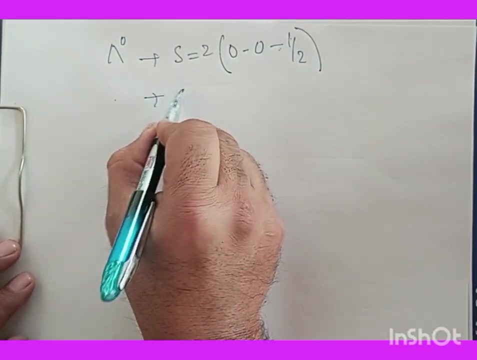 doesn't have the third component of isospin and its period number is: we have here minus one by two, using for B equal to one. so what will be the strangeness for this particle? this will be plus, this will be no, this will be minus one. 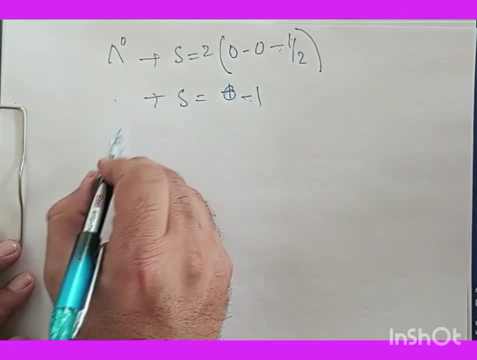 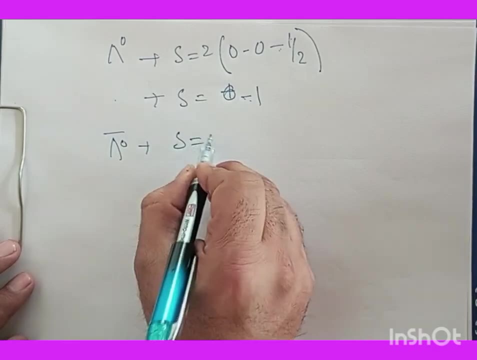 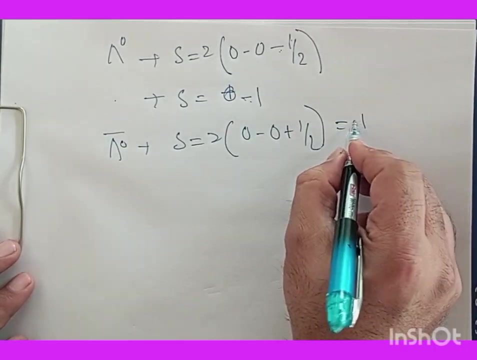 minus one, and we can take on another particle, say, say, the anti particle of this, this lambda. for that the strangeness will be two times. it is zero minus zero. here I'll have plus one by two. so this is going to give me the plus one. and now say, for example, I will take a proton, and and proton is not a strange. 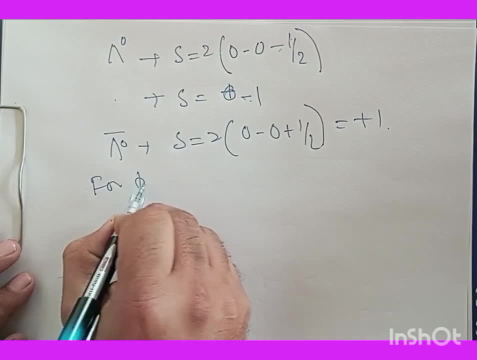 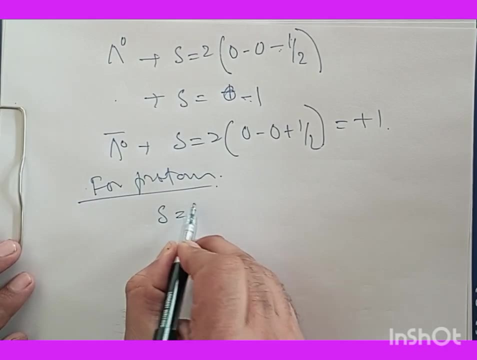 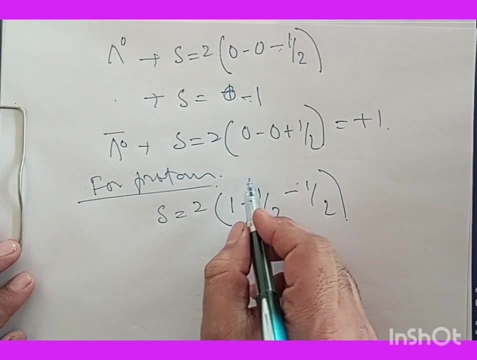 particle. so for proton, I'll use the same formula for proton. what am I going to get here is is that the strangeness will be two times yeah, what's its charge is one, and its third component is is one by two, and this will be minus one by two. okay, so we can see that this whole thing is going to die. 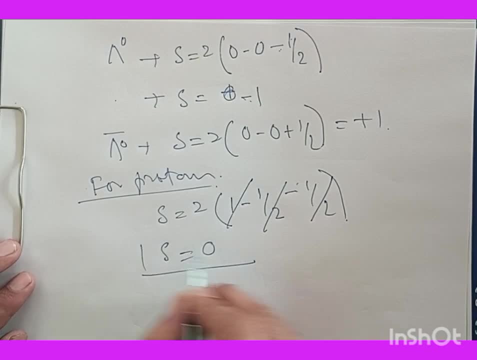 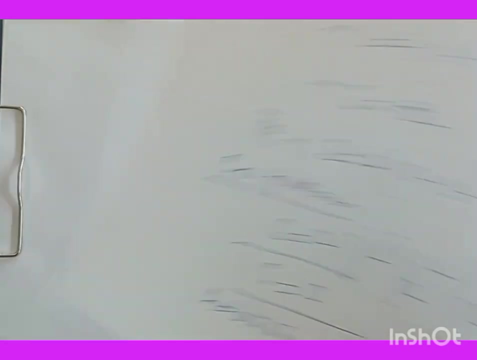 and strangeness, for this is going to be zero. and this strangeness, quantum number. it is a additive in nature, it is additive in in nature. now, let's, let's talk about, let's talk about. so here we have, we have talked about this strangeness, quantum. 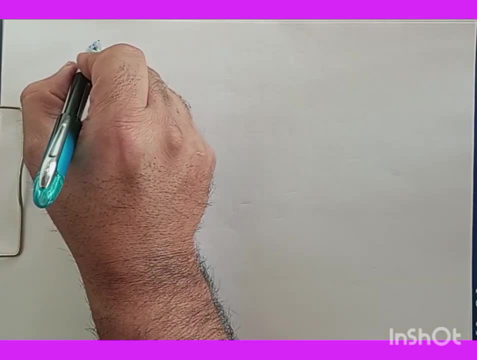 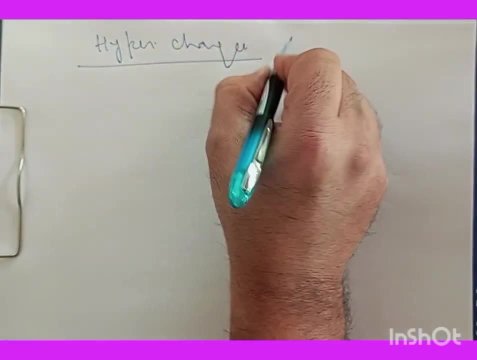 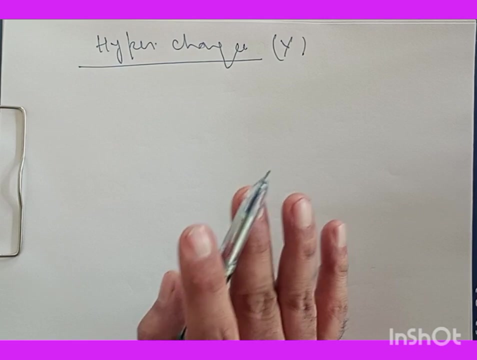 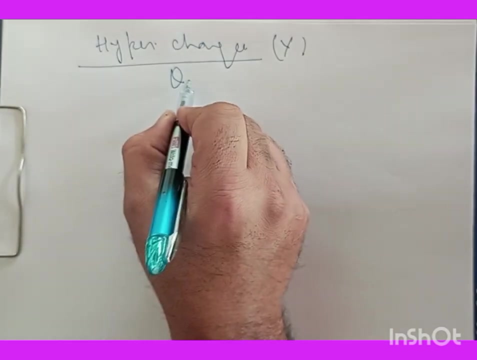 number. now let's talk about this hyper charge. hyper charge, hyper charge. why? why now, this hyper charge quantum number? it is basically defined as as twice the once hyper charge quantum number. it is basically defined as is twice the average charge of each particle group. so so if I have Q charge, then the, the, 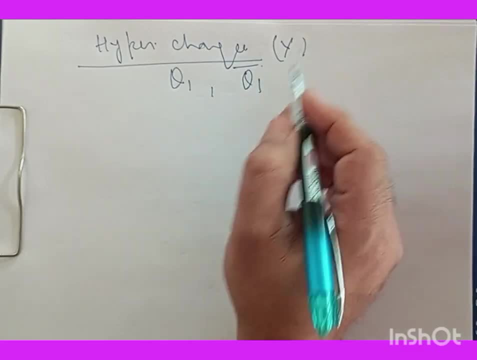 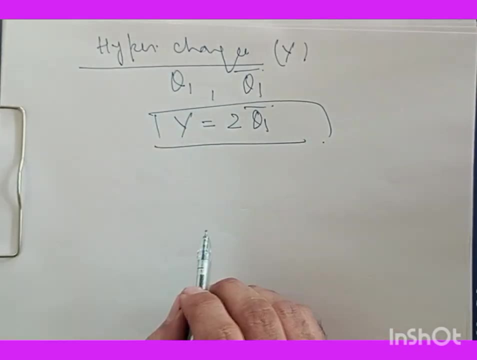 average of this character is Q1 bar. so this hyper charge is simply two times Q1 bar. so this hyper charge is simply two times Q1 bar now, for example, two times q 1 bar. now, for example, if I take a nucleon group of proton and neutron, say, for example, and if I take a proton and 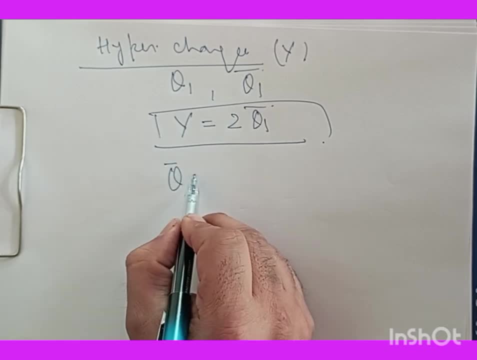 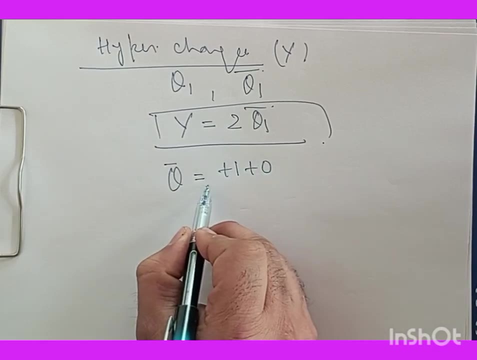 neutron as a group. what will be Q bar for that It will have. the charge of proton is plus one and there is no charge for neutron divided by two. So this is going to give me one by two. So what's going to be the hypercharge for this system is twice Q bar, So this is two times one. 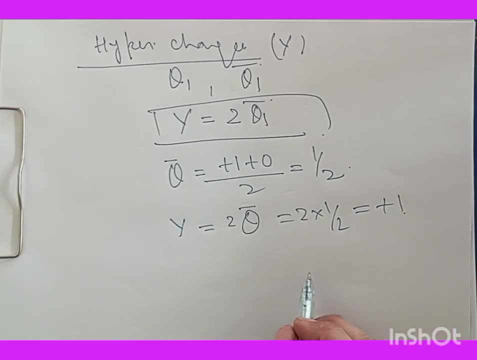 by two and this will give me plus one. Now, as we already know that this Q bar is, it is, it's Q minus no, not twice, it is Q minus I3.. We have a relation between this Q bar and Q. 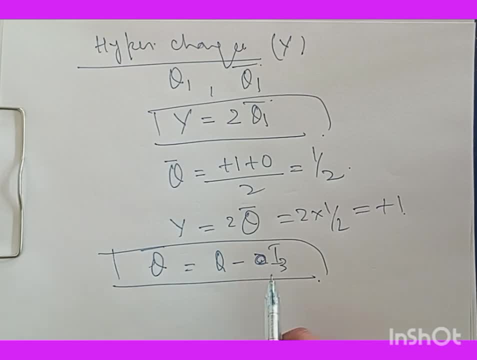 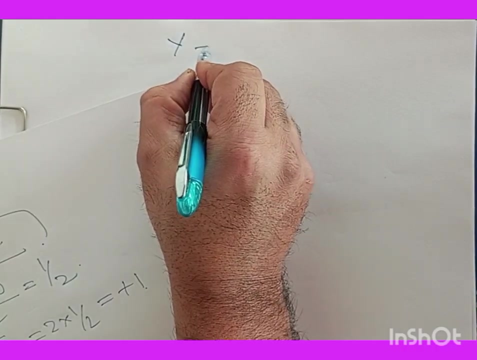 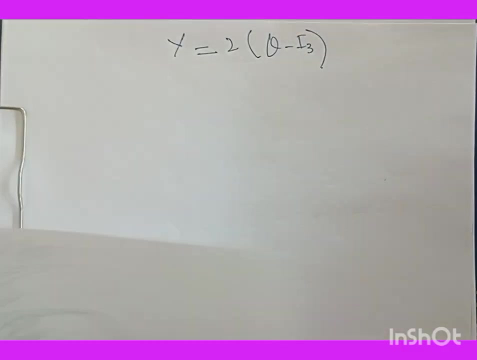 as Q minus I3. So if this Q bar is Q minus I3, I can use this here in this equation. now, if I use it here, what am I going to get? I will get? this hypercharge is two times Q minus third component or third coordinate of isospin. 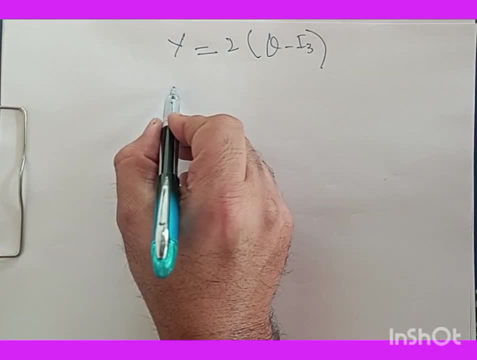 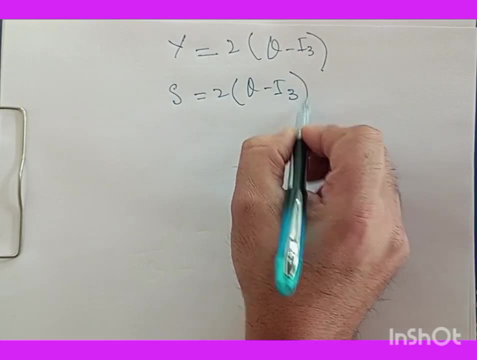 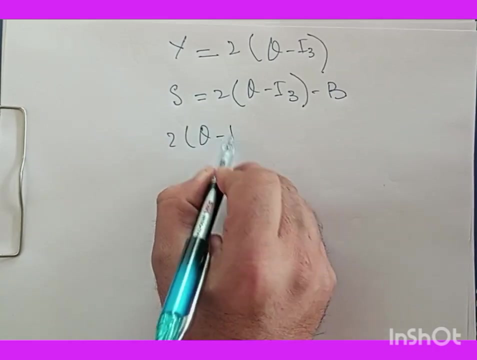 This will be the case And we already know that strangeness S is it is two times Q minus I3 minus B. So from this equation I can have: two times Q minus I3 is this: S will stay, this minus B will become plus B. 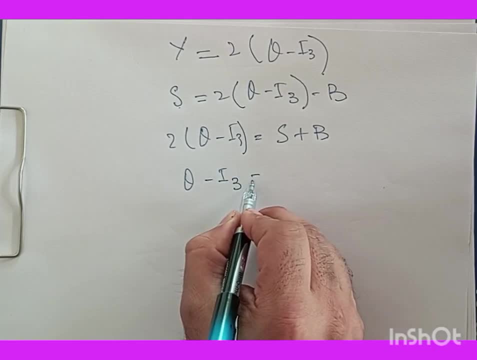 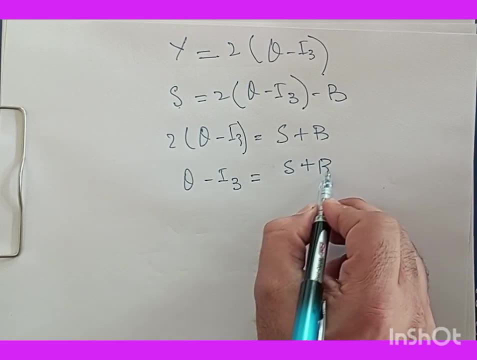 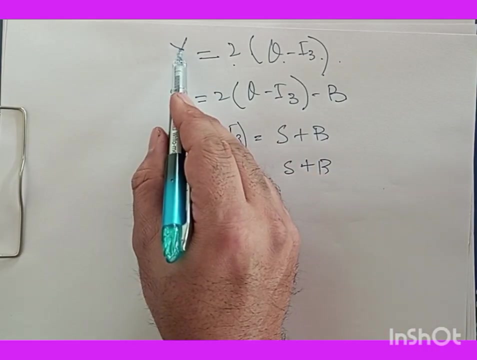 So Q minus I3 is going to be S plus this is S plus B. twice of this And we already have two times Q minus I3 is already equal to hypercharge. So from this equation I can have two times Q minus I3. is this: S will stay, this minus B will become plus B. So from this equation I can have two times Q minus I3. is this: S will stay, this minus B will become plus B. So from this equation I can have two times Q minus I3. is this: S will stay, this minus B will become plus B. 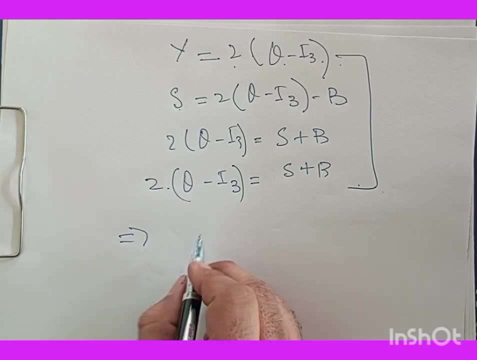 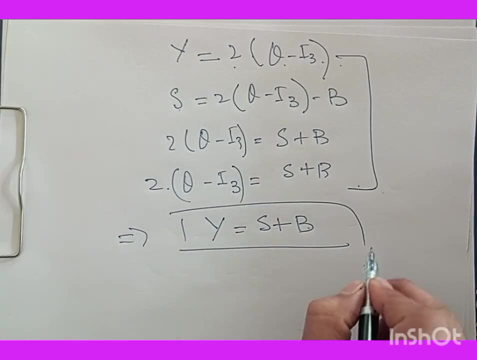 So we can have, we can equate the two equations and we will get this hypercharge equal to strangeness number plus baryon number. And similarly we can calculate the hypercharge of different electrons, mesons, nucleons and hyperons based on this equation. 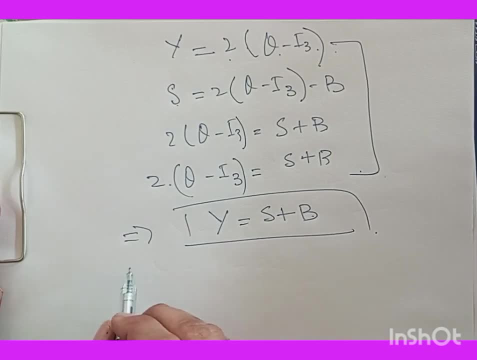 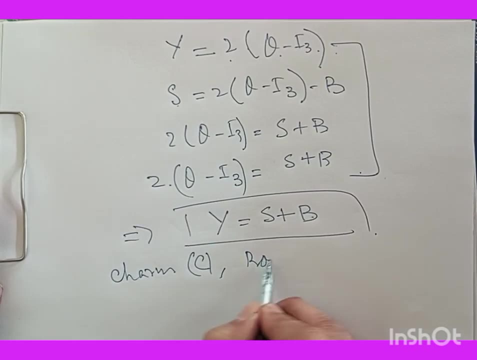 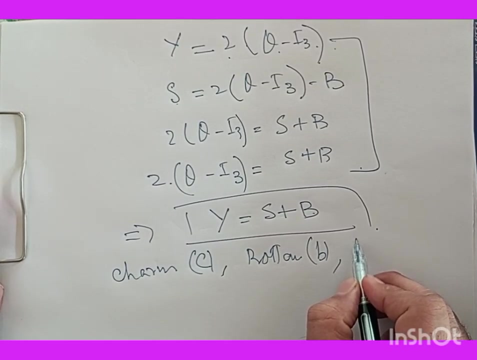 And there are three additional quantum numbers, like one is called charm, and it is symbolized as C, then we have bottom and it is symbolized as B, and then we have up- no, it's not up, it's top- and it is symbolized as T. 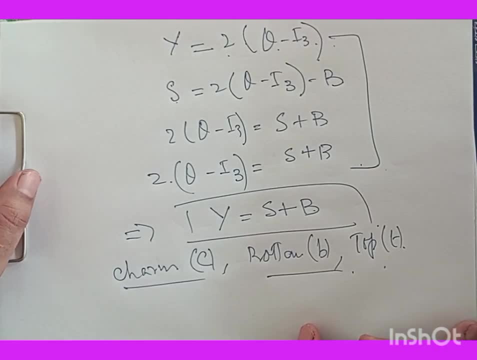 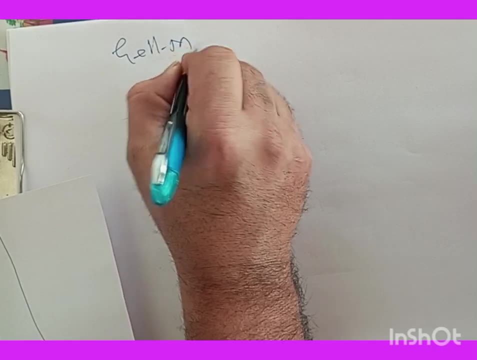 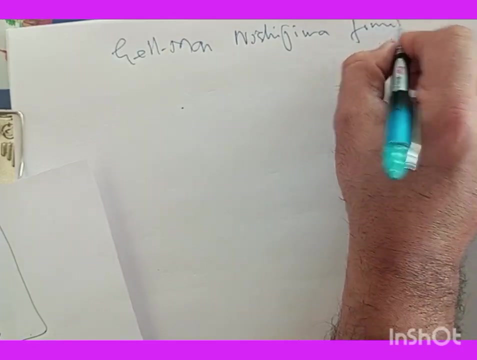 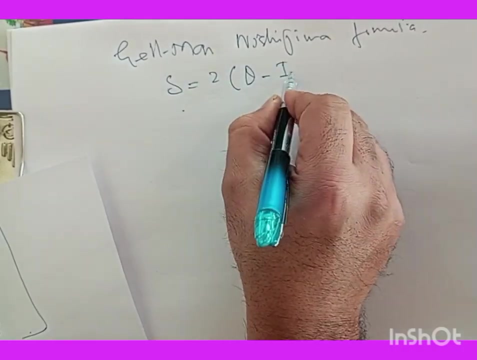 Now this Gell-Mann-Nishijima formula. this formula is given by what We have: Gell-Mann Nishijima formula. What is that? That formula is that this S is two times Q minus third component of Iso-Spin minus B. 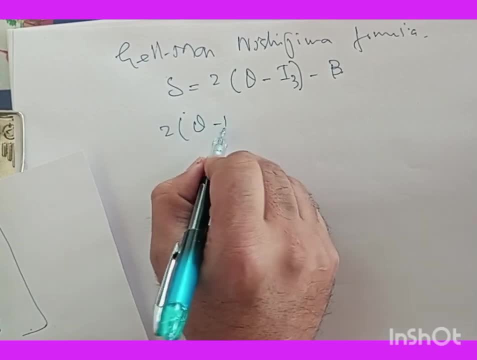 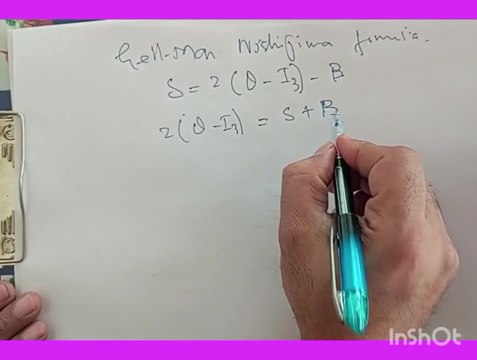 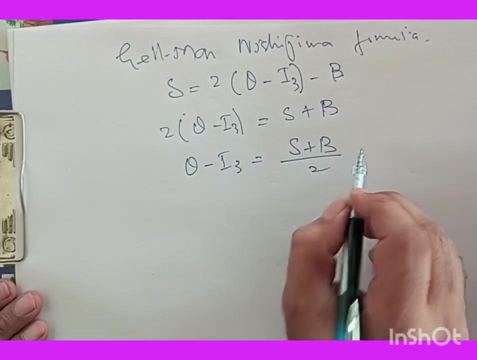 Or from here: if I write two times Q minus I3 is S plus B, nothing wrong with this. And this Q minus I3 will be S plus B divided by 2. And I can calculate this charge as I3 plus S plus B. 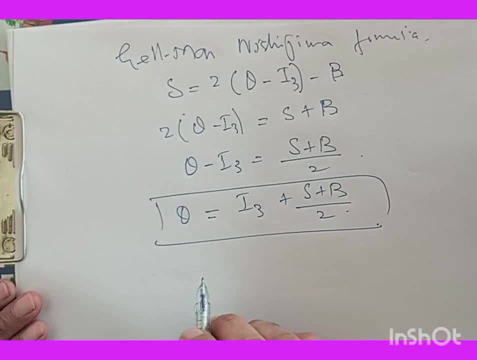 divided by 2.. Now, with the discovery of the new elementary particles, I mean the quantum numbers, like charm, bottom, top, these quantum numbers were explained and they were introduced to explain the properties of these new particles And the introduction of these new quantum. 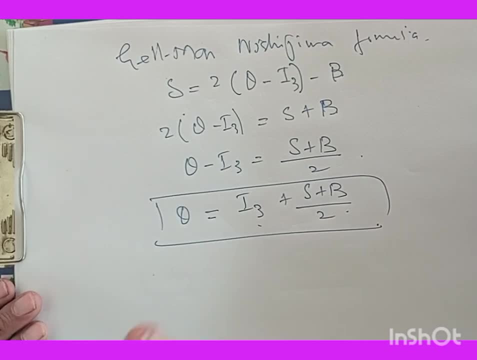 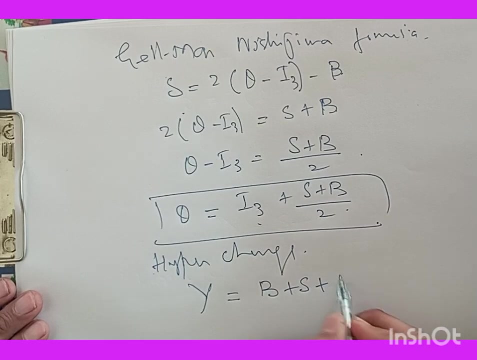 numbers. I mean this hypercharge that we have, which is hypercharge, as we have that Y, that Y is, it is B plus S. Now the other quantum numbers are added to it, plus charm, plus top, plus bottom, And accordingly we will have: 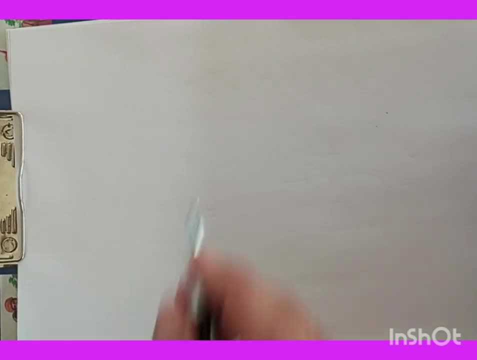 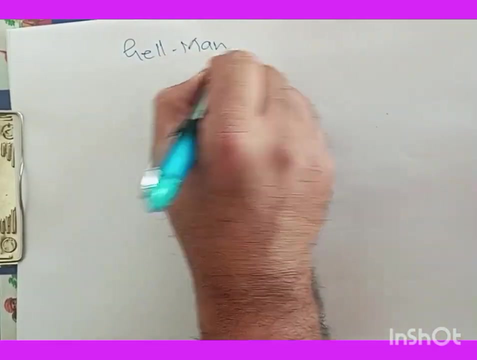 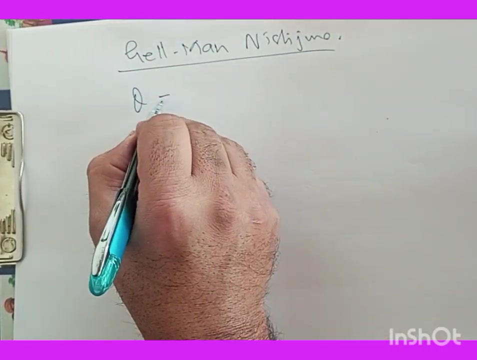 So we will have this Gell-Mann-Nishijima formula modified, And what will be that formula? This Gell-Mann-Nishijima Okay, So that will become: Q is I3,. we have okay plus B.